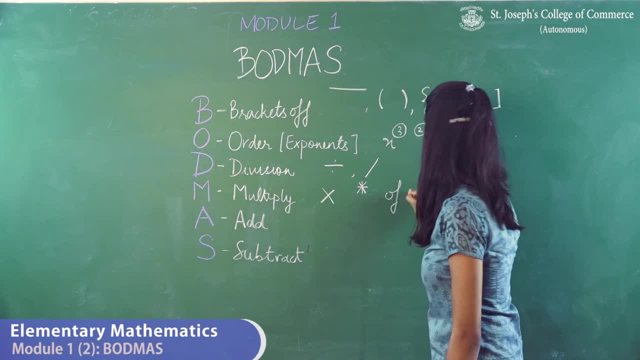 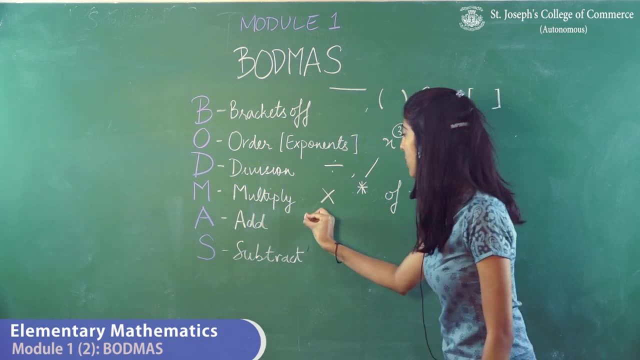 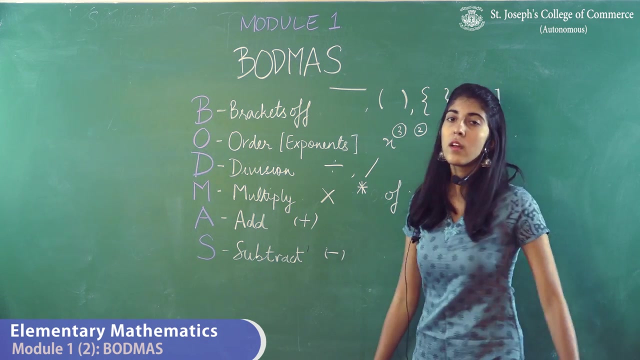 Or the asterisk, Or it is said to be represented by the word of A stands for. add Addition sign can be represented only by the plus sign, And subtraction sign, which is what S stands for, can be represented by the negative sign. 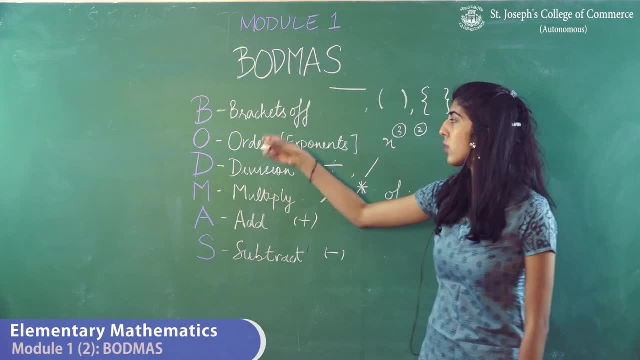 When you're solving sums under Bored Mass, you need to ensure that you follow this order in order to get your right answer. So you start off by removing the brackets, Then you start off by removing the brackets, Then you start off by removing the brackets. 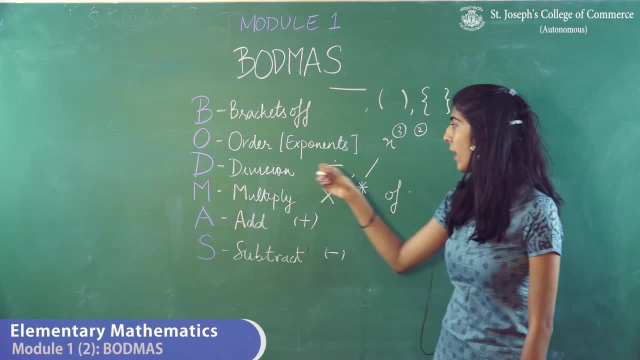 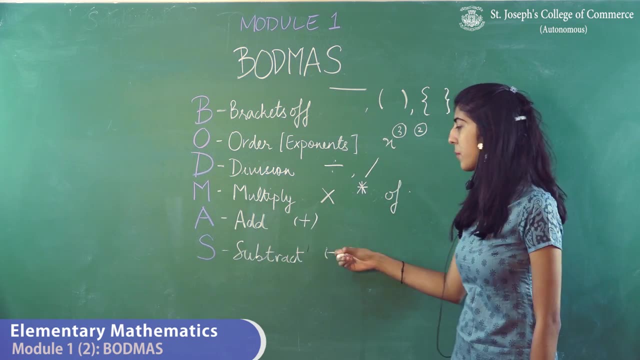 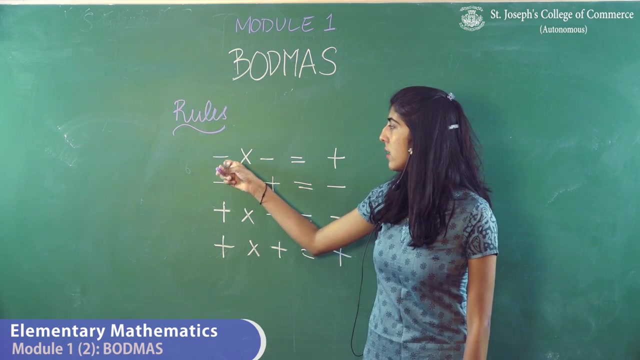 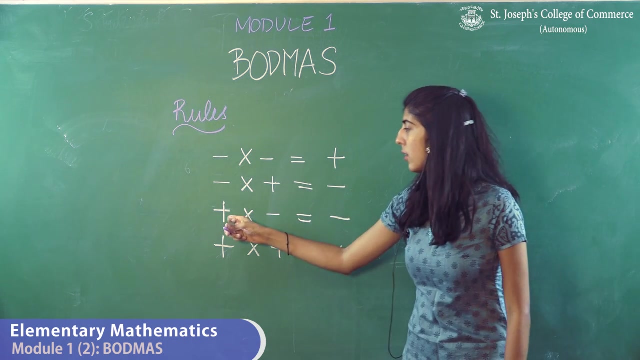 Then you start off by removing the exponents, Solving the exponents, Then dividing anything that needs to be divided, Multiplying the terms, Add any terms that have a plus sign attached to it And then subtract the set terms. Certain rules to remember before solving sums under Bored Mass. The first rule is: minus into minus will give you plus. Second, one is minus into plus will give you minus. Third, one is plus into minus will give you minus. And the fourth one is: plus into plus will give you minus. 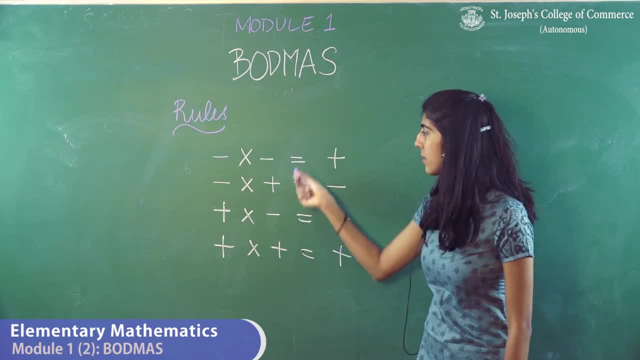 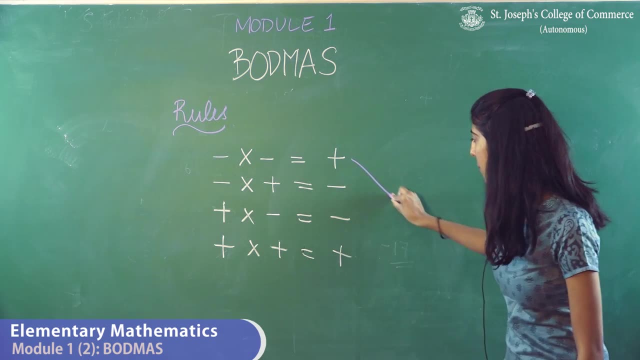 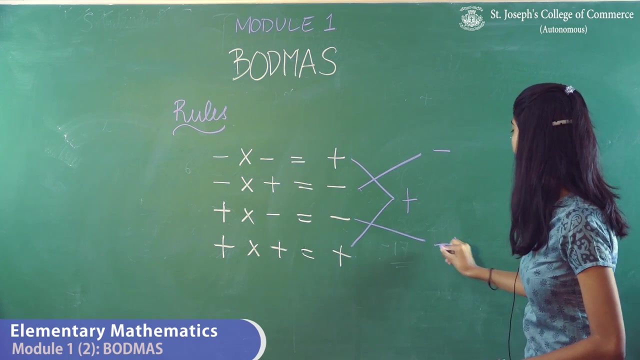 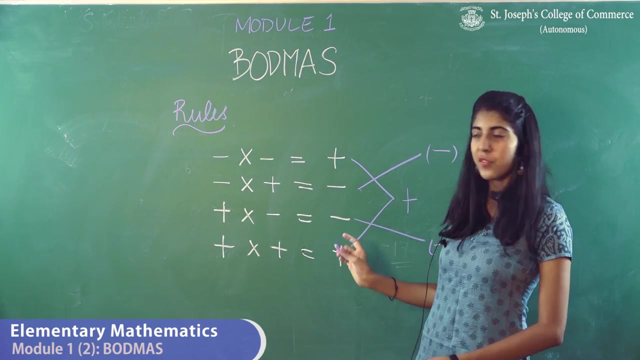 If you notice, same signs, when multiplied, will give you an addition sign And opposite signs, when multiplied, will give you a negative sign. So same signs, positive, negative, These are opposite signs, No matter what order they are in. if opposite signs are multiplied, they will give you a negative sign And if same signs are multiplied, they will give you a positive sign. 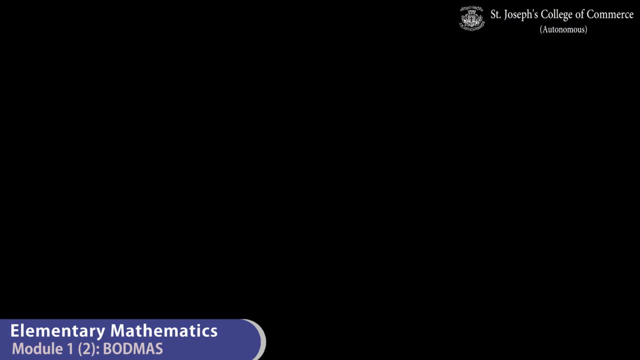 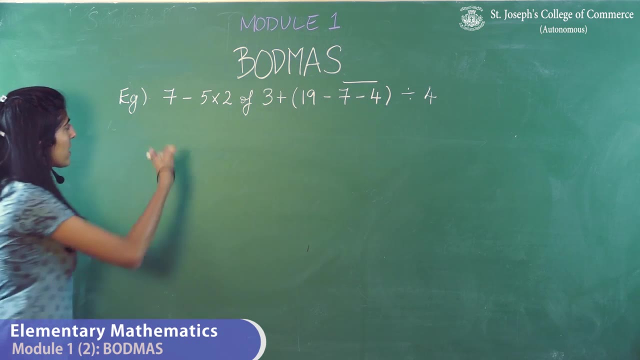 Lets move on to solve the sums. Lets move on to understand how to solve a sum using Bored Mass. This is an example of a sum: 7 minus 5 into 2, of three plus 19 minus 7 minus 4 divided by 4.. 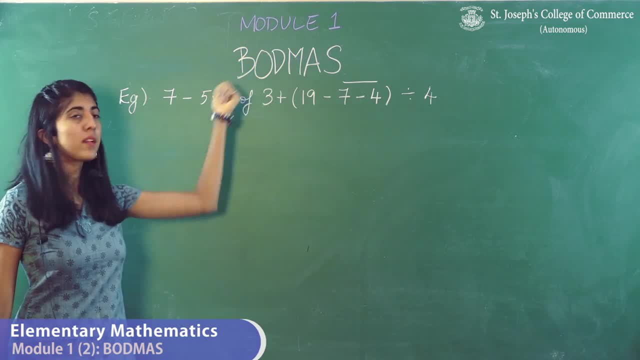 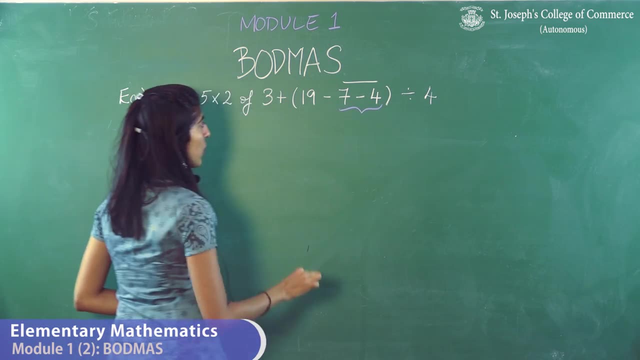 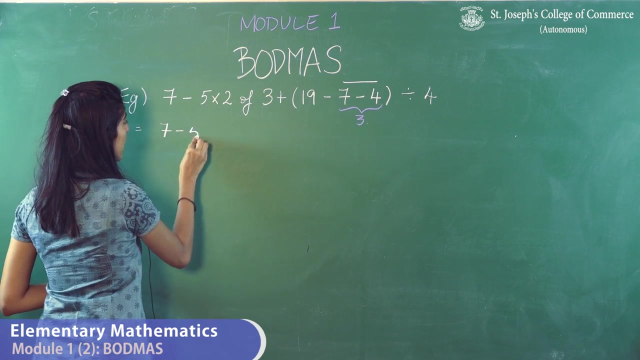 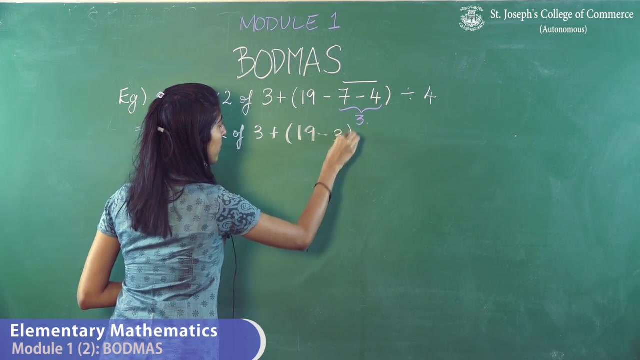 So you start with the first thing. The first letter under Bored Mass is B, so you try to eradicate the brackets. The first bracket you need to remove is the bar bracket, So you will solve this first. 7 minus 4 is 3.. So when I solve it I need to rewrite the whole thing as 7-5 x 2 of 3 plus 19-3 divided by 4.. 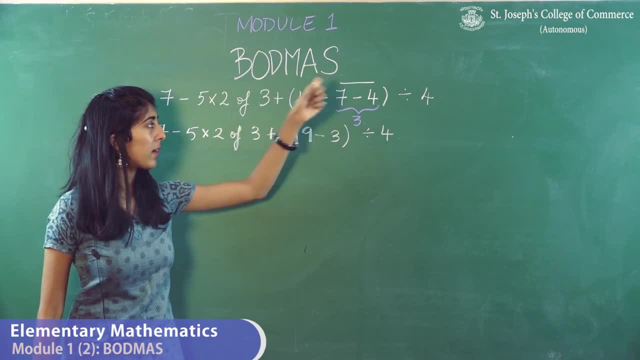 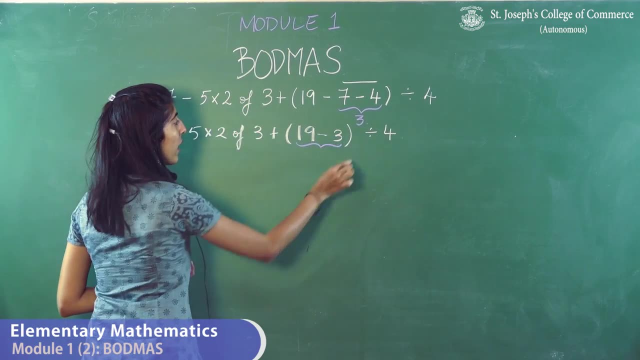 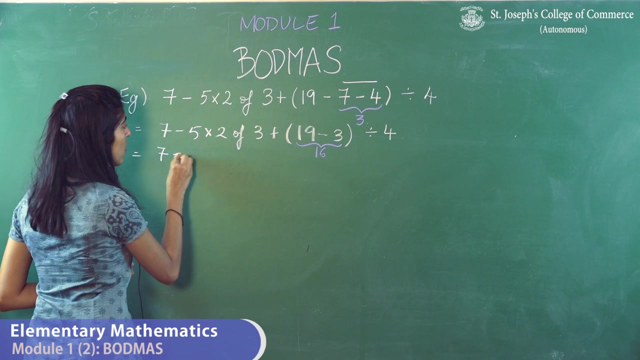 Okay, We've only taken out the bar bracket. The next bracket under brackets are curve brackets, So the next step would be to solve whatever is inside the curve bracket. 19-3 is 16.. So the next step would be to rewrite the whole equation: 5 x 2 of 3 plus 16 divided by 4.. 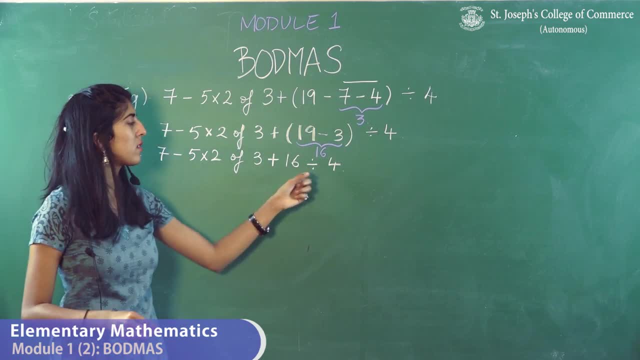 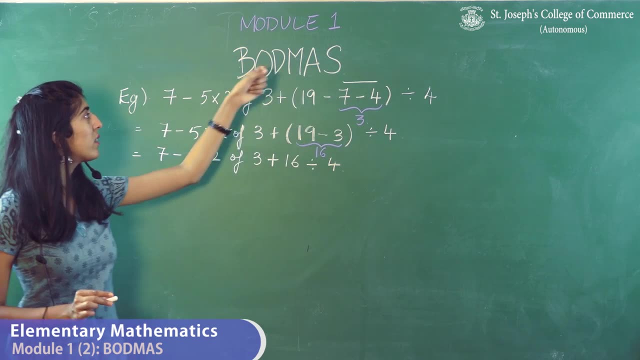 If you notice, I've just removed the brackets and just written the direct answer as 16.. You don't need to include the brackets here. The next thing to do: b is over, o isn't there in the sum. The next thing is to do is division. 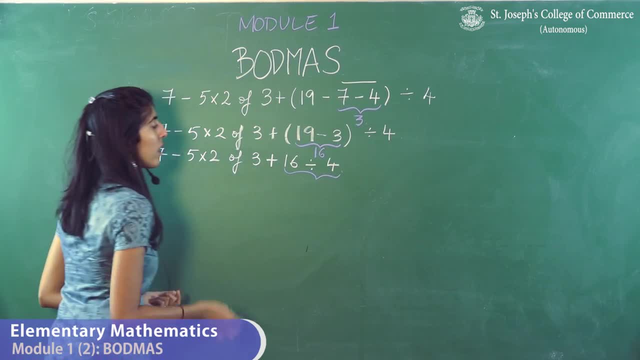 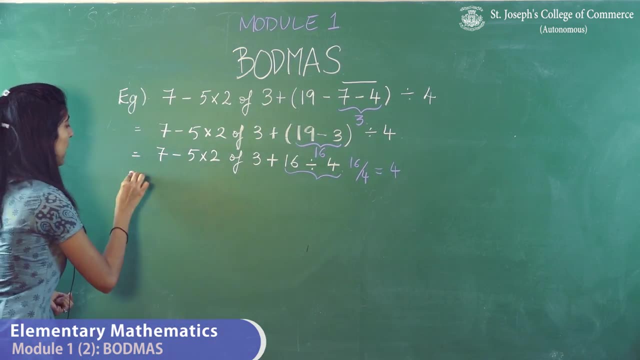 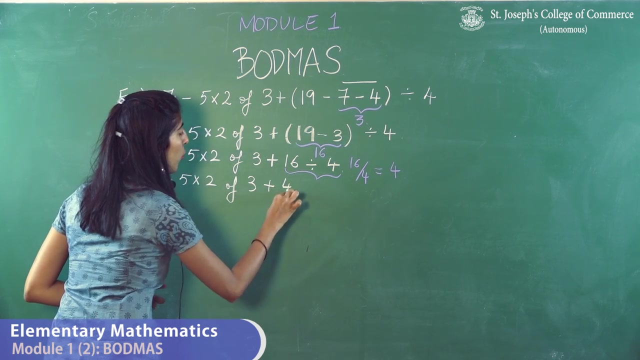 If you notice, only 16 by 4 has a division sign. So you do 16 divided by 4, which is equal to 4.. So when I rewrite the next step, it will be 7-5 x 2 of 3 plus 4.. Again, I'm repeating: you solve 16 divided by 4, because division is next. 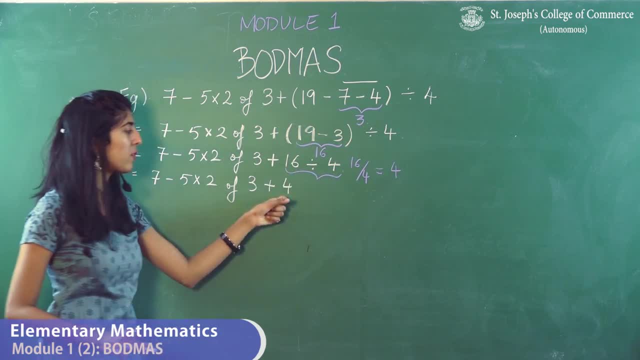 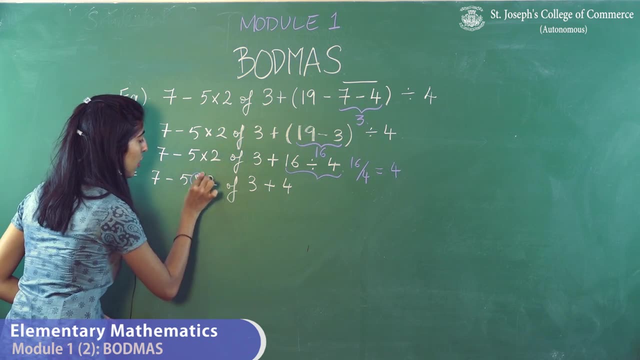 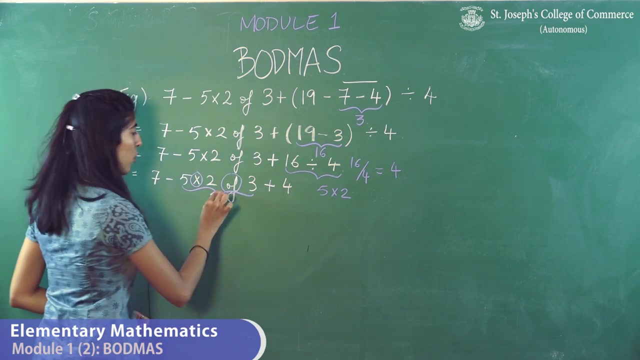 So 16 divided by 4 is 4.. So I just rewrite this part as 4 in this equation. The next thing to do would be to multiply. If you notice, here this is also multiplication and off is also multiplication. So when I solve 5 x 2 x 3, I get the answer as 30.. 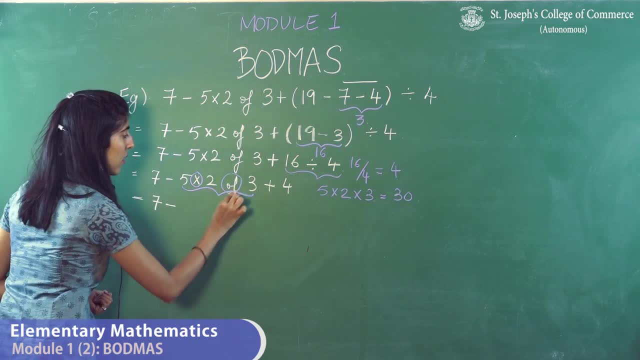 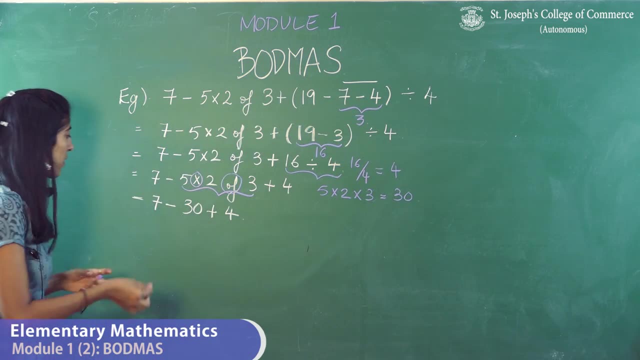 So when I rewrite the equation again, it will be 7-30 plus 4.. Next thing to do would be to add. If 7 does not have any sign preceding it, it is assumed to be positive 7 plus 4.. So I add it first. So I do 7 plus 4.. 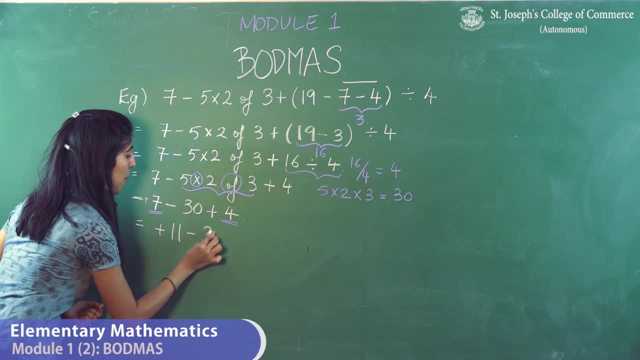 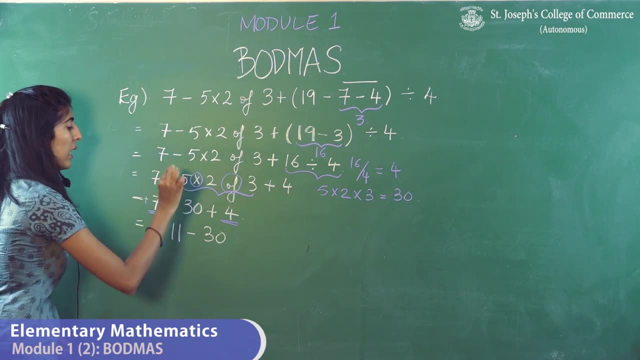 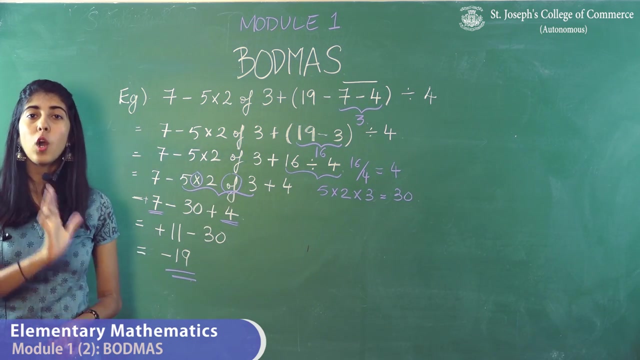 7 plus 4 is plus 11 minus 30.. Next thing to do would be to subtract Plus 11 minus 30 is minus 19.. Therefore, this is your answer, Solving it by any other way, By just mixing division multiplication. 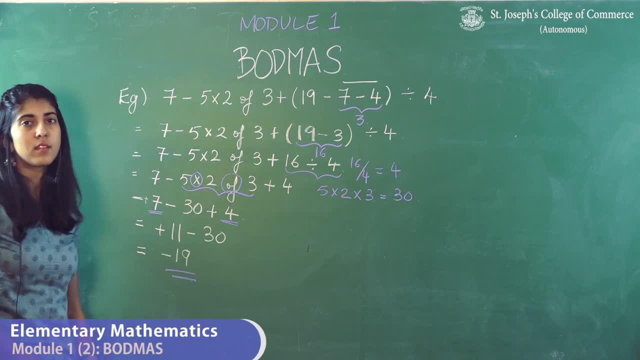 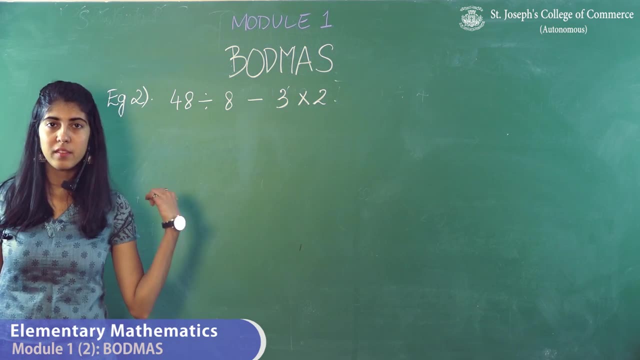 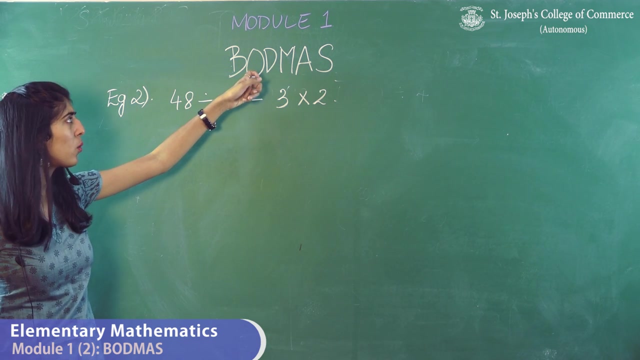 Addition and subtraction up would not result in this answer. We're going to try solving a different example: 48 divided by 8 minus 3 into 2.. If you notice, there are no brackets, there are no orders, So you directly start off with starting with division. 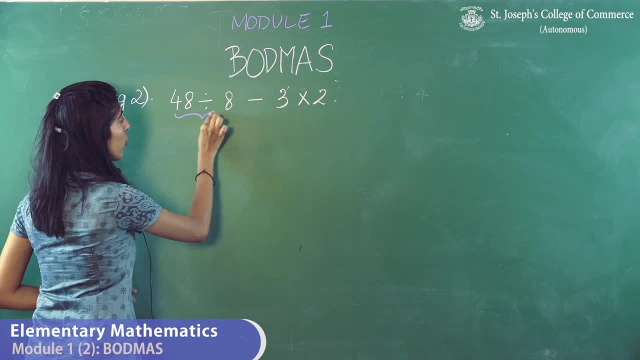 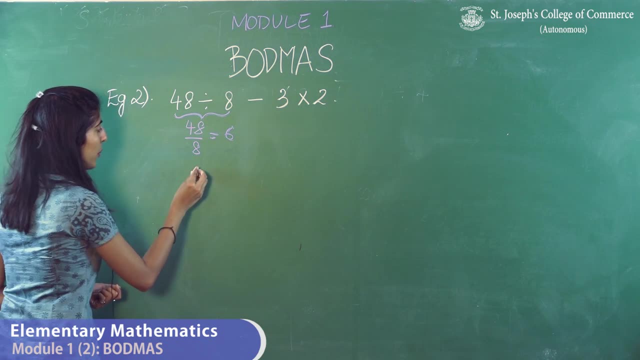 So, if you notice, only division has only 48 and 8.. So I solve this first: 48 divided by 8 will give me 6.. So the next step would be to write 6 minus 3 into 2.. 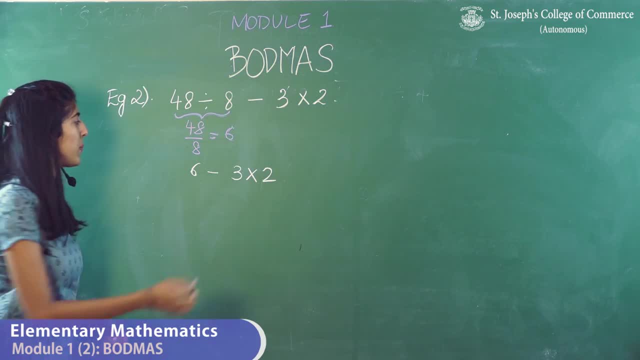 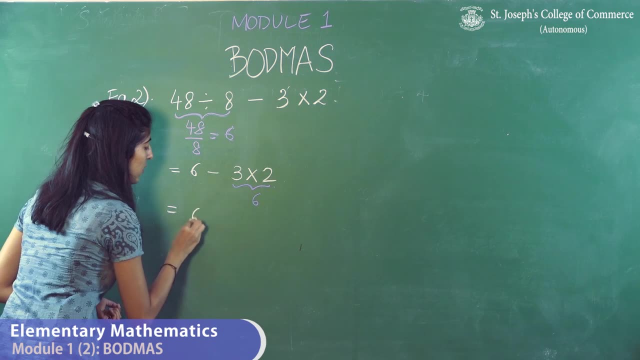 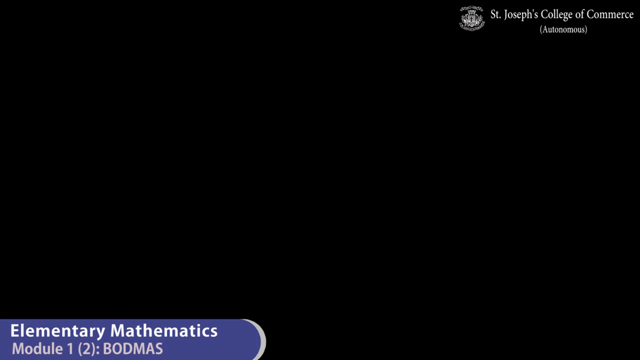 As division is already solved, we move on to multiplication. Multiplication is only 3 into 2, so that is 6 as well. So the next step would be 6 minus 6, which is directly 0.. We're going to solve another sum under BODMAS. 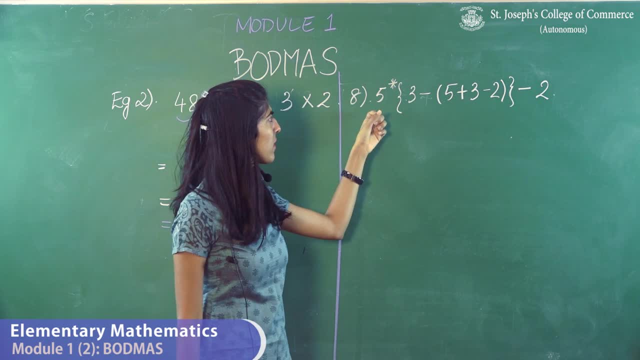 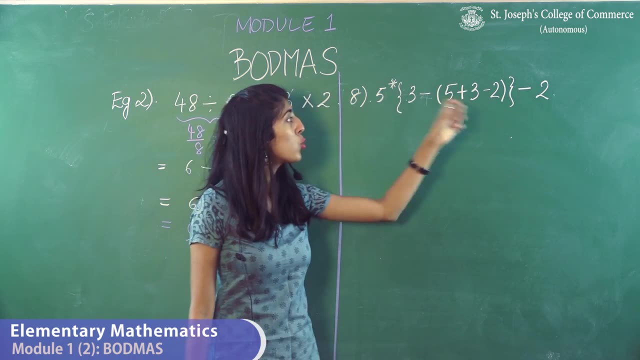 This is the 8th sum in the handout. The sum has 5 into 3 minus 5 plus 3 minus 2, minus 2.. If you notice, there are 2 brackets and there's no bar bracket. 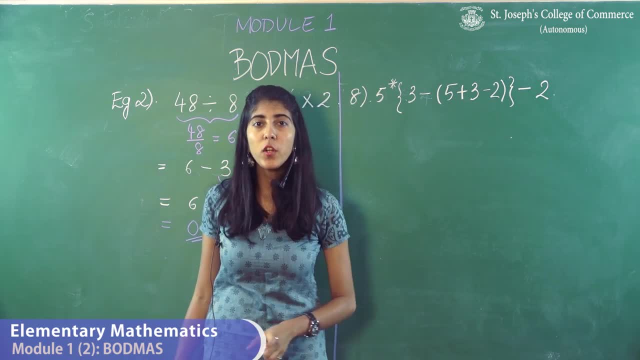 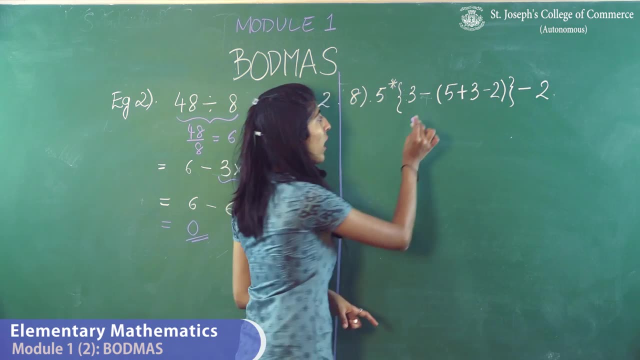 So you start off by solving the curve bracket. Another important thing to remember is, when you're solving anything inside the bracket, you need to utilize BODMAS as well. So under this there are only plus signs and minus signs. So you start off by adding: because a comes before the a. 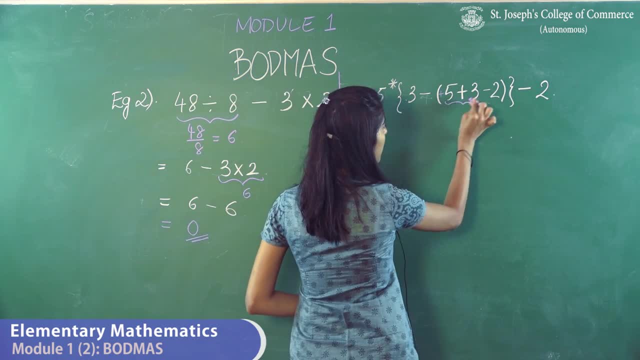 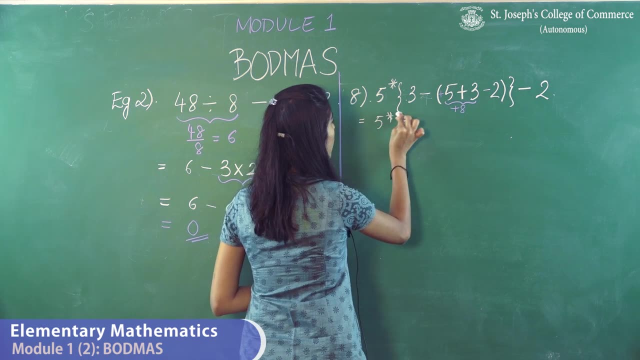 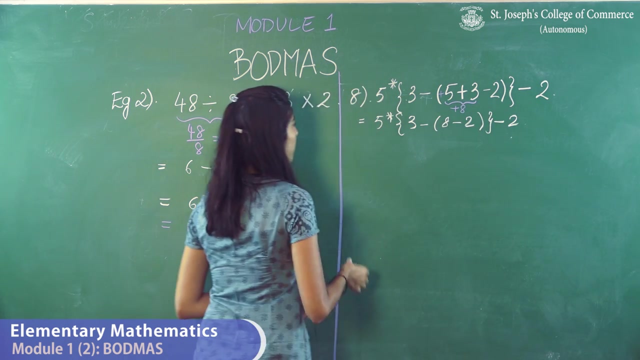 So you start off by adding because a comes before the a. So you start off by adding because a comes before the a. So when I add it, this becomes 8, plus 8.. So when I rewrite the thing, it'll be 5 into 3 minus 8, minus 2, minus 2.. 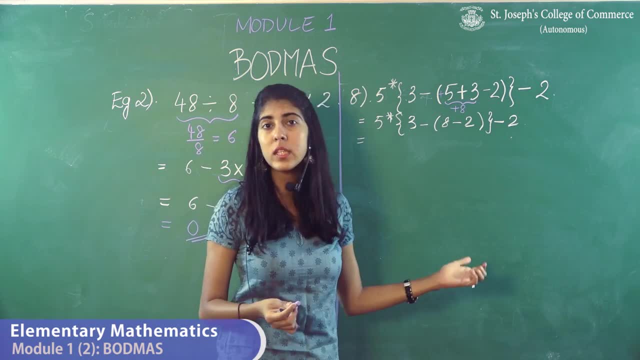 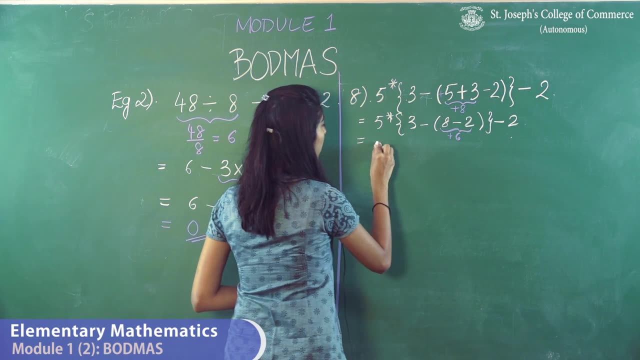 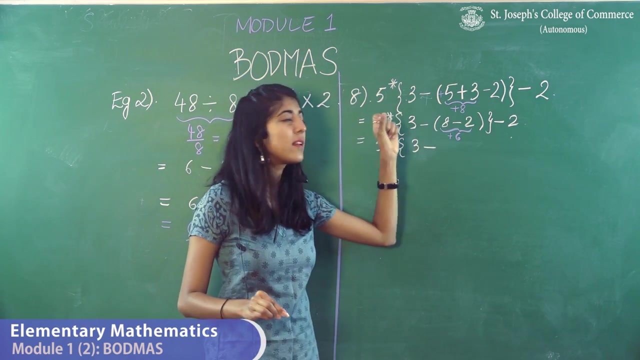 The next thing would be to just subtract 8 minus 2, because there's no other thing inside the bracket. So this would be 6, but it is plus 6.. So when I write 5 into 3 minus, you need to remember that outside the bracket there's a minus sign.